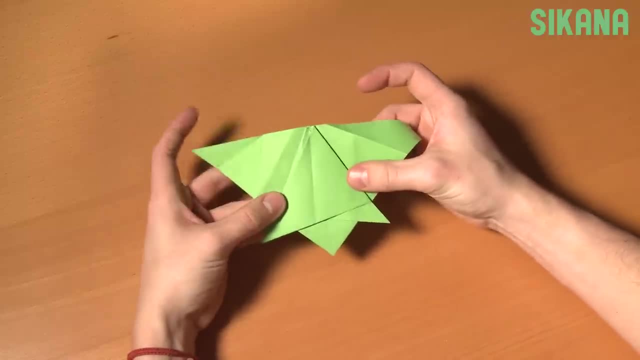 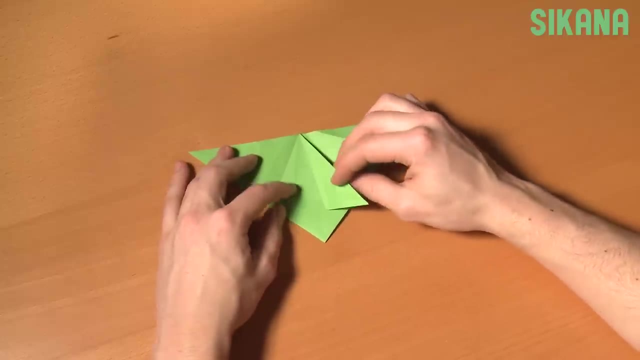 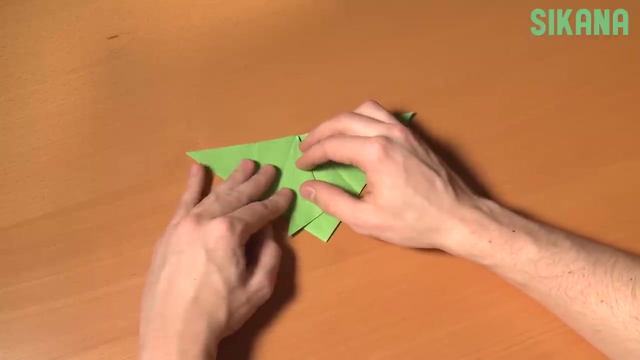 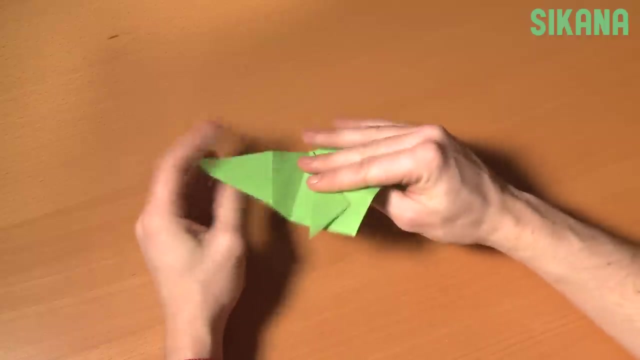 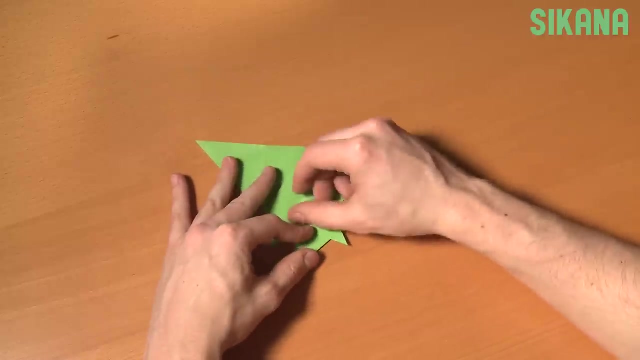 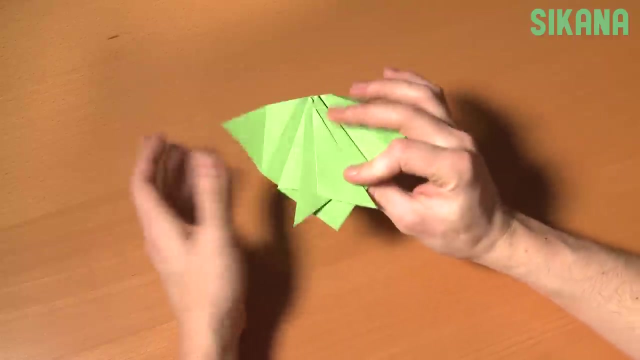 Fold it diagonally. Fold it in half. Fold it diagonally. Open this part and fold this side over the fold. This will create the fin which sticks out here. Fold on the other side to make the other fin. Both fins should be the same size and you should get this shape. 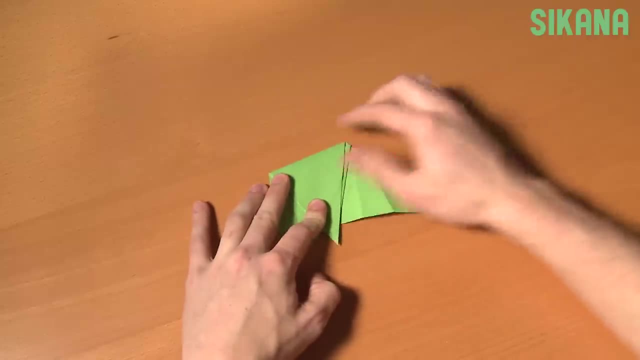 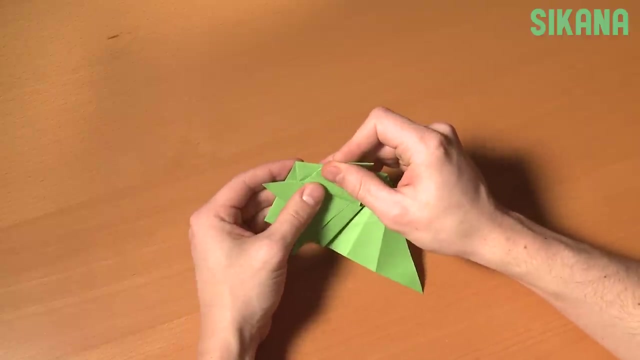 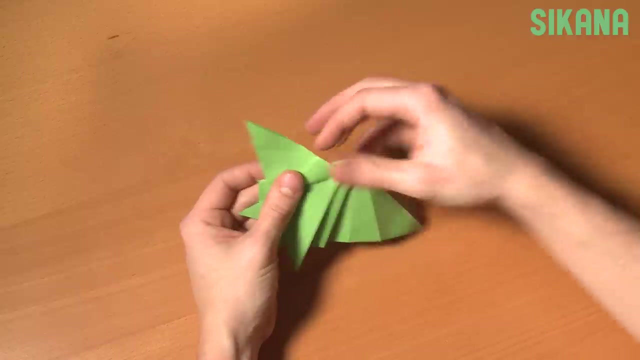 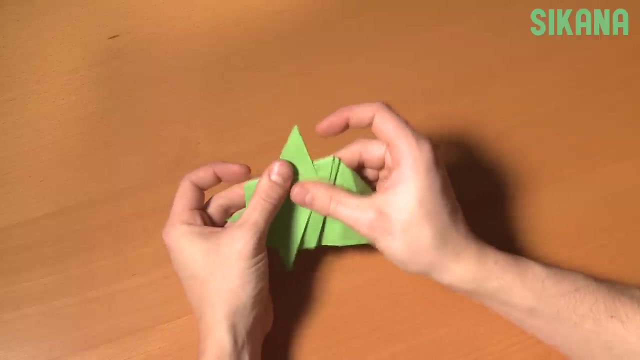 Now fold this part over as far as possible like this, Then fold in the opposite direction down to here. Slide the fold slightly to allow the top of the triangle to stick out perpendicular to this side like this. Now for the third fin. 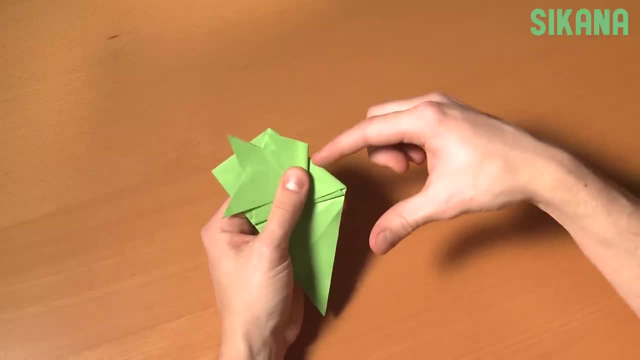 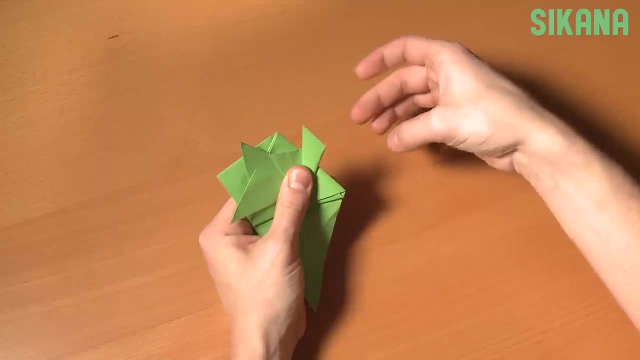 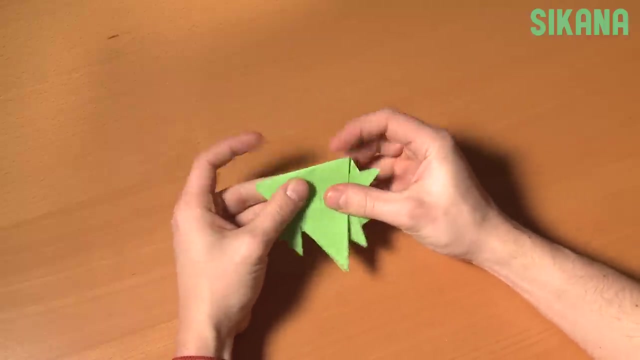 Fold in the opposite direction and slide the fold until this part is parallel to this one. Now repeat this step on the other side. Fold this part over as far as possible. Then fold it in the opposite direction up to the mark. 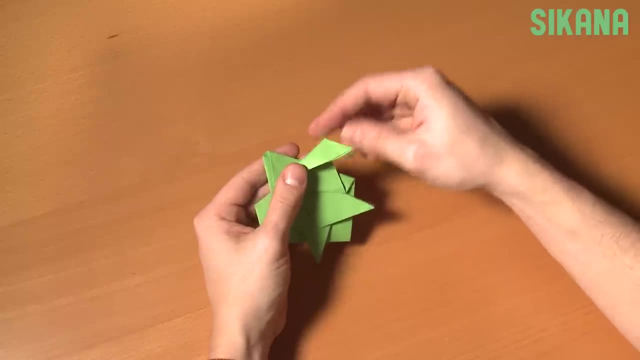 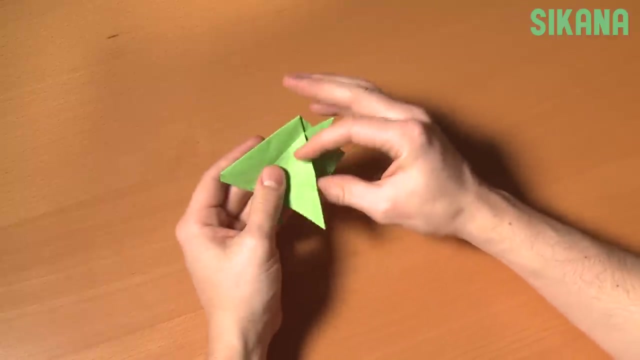 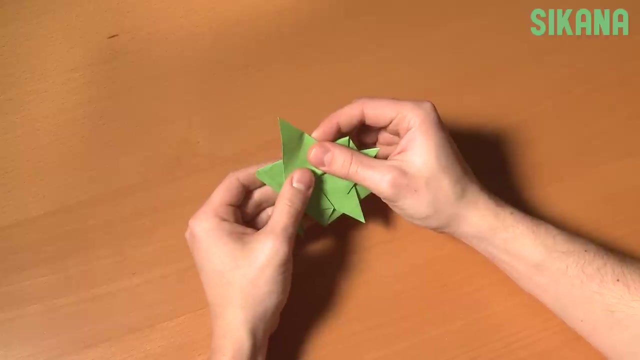 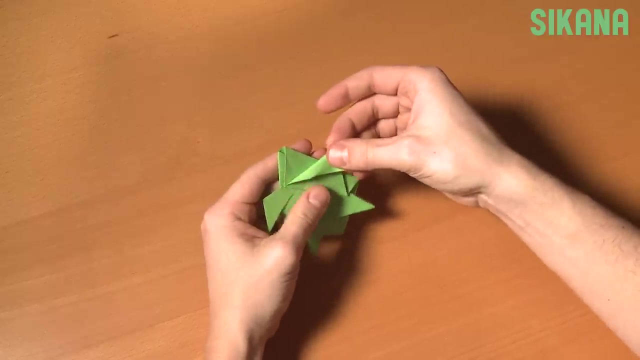 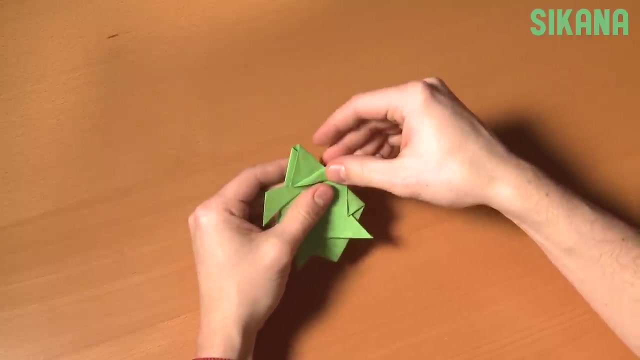 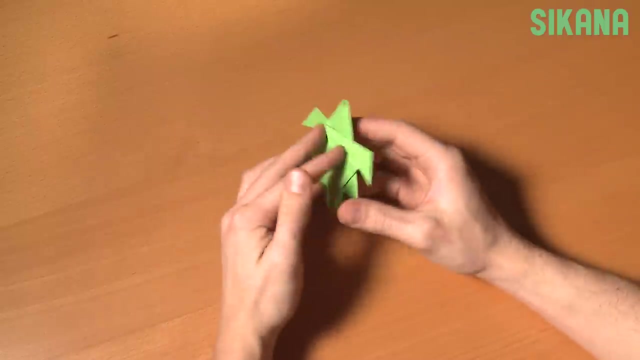 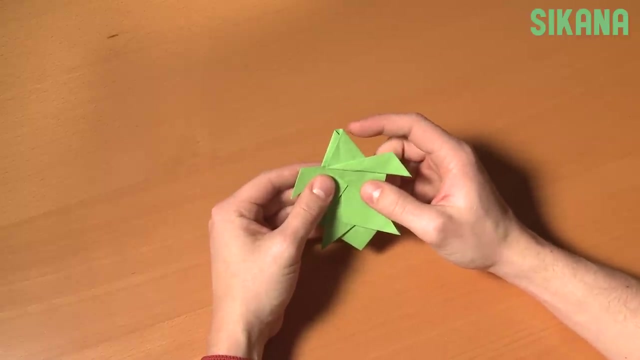 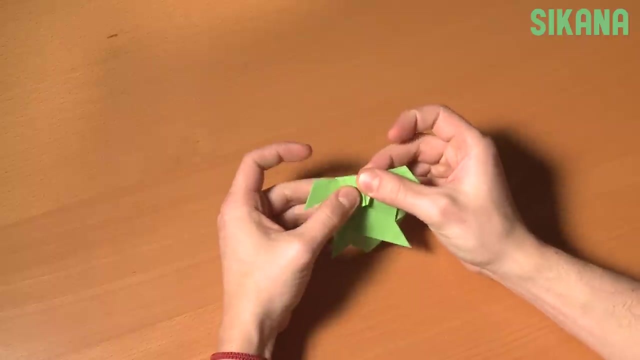 Fold this part down and try to make a triangle. Make it as long as the other side, Then fold it in the opposite direction up to the mark. Let's move on to the head. Fold this part downward once, Then fold it upward, making sure to leave some space. 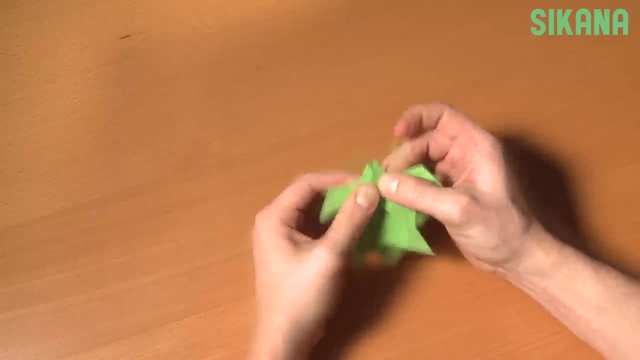 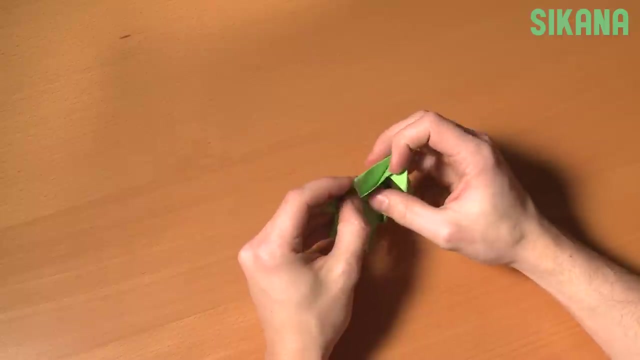 Then fold it down once. Then fold it back up, making sure to leave some space. Then fold it up, making sure to leave some space. Finish up the shell to complete your Turtle Origami. For this step, fold the lateral extremities under the shell like this: